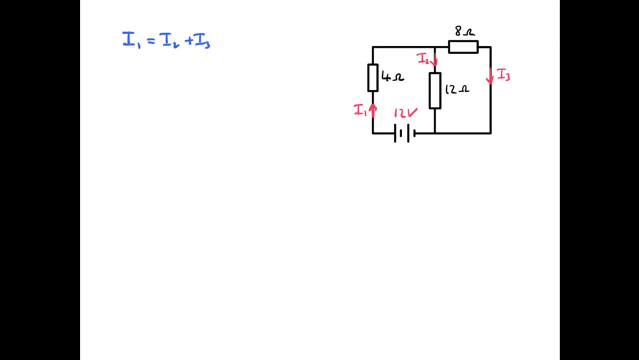 Okay, so here's my solution. Well, firstly, if you look at the junction at the top there, you can see I1 is going into that junction and I2 and I3 are going out, So we can state that I1 is equal to I2 plus I3. 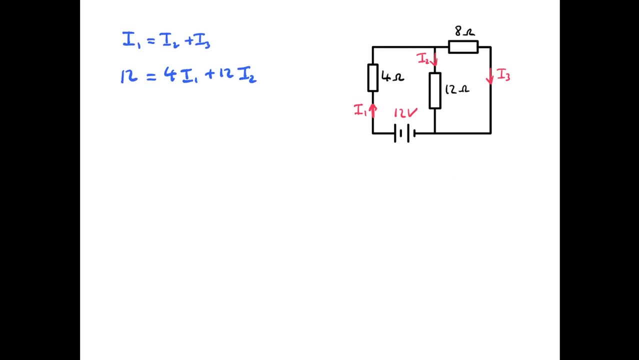 And if we look at the loop on the left-hand side, well we know the 12 volts the EMF going in must be equal to 4I1 plus 12I2.. If we look at the outside loop, we can see that 12 volts the EMF from the battery must equal 4I1 plus 8I3.. 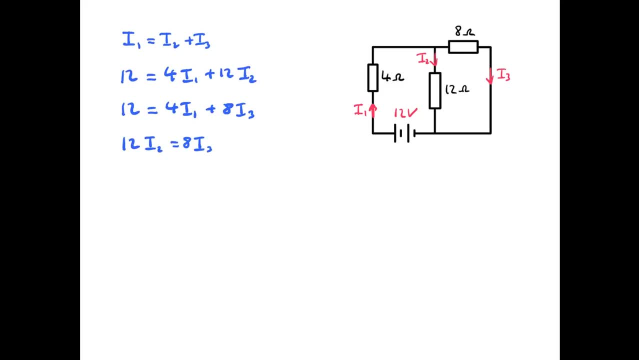 Now, with this information, we now know that 12I2 must equal 8I3.. Now let's try and work out what's the total resistance of our circuit. Well, firstly, we've got the 12 ohms and 8 ohms. Although it might not appear like it, they're actually in parallel. 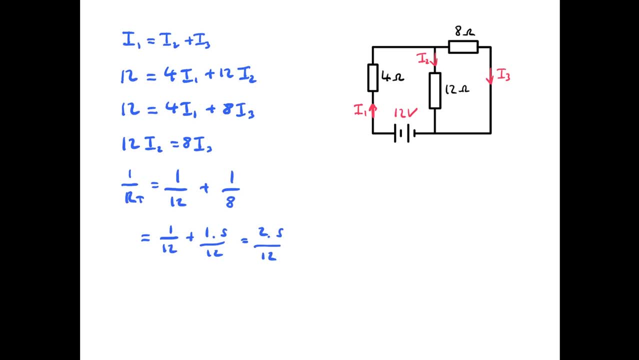 So we can work out what their total resistance is. Okay, So we can work out that the total resistance of the 12 ohms and the 8 ohms in parallel is actually 4.8 ohms. And add that to the 4 ohms on the left, we get a total resistance in our circuit of 8.8 ohms. 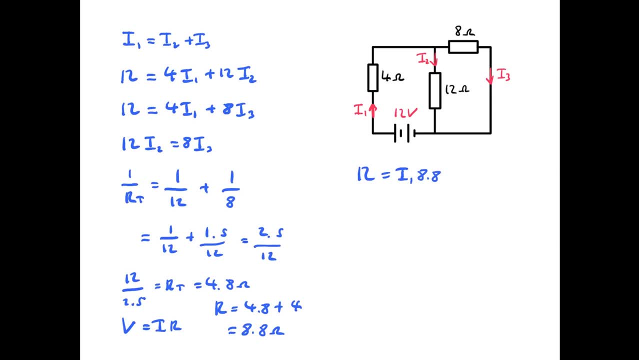 Now we're going to apply: V equals IR, So we know that 12 is equal to I1 times by 8.8.. So therefore, I1 is equal to 1.36 amps. We can just substitute our values for I1 into our equations at the top left-hand side. 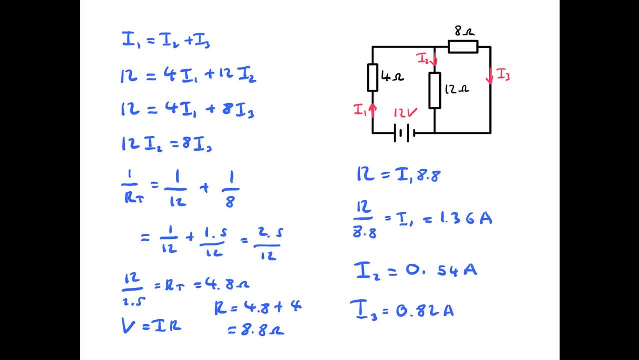 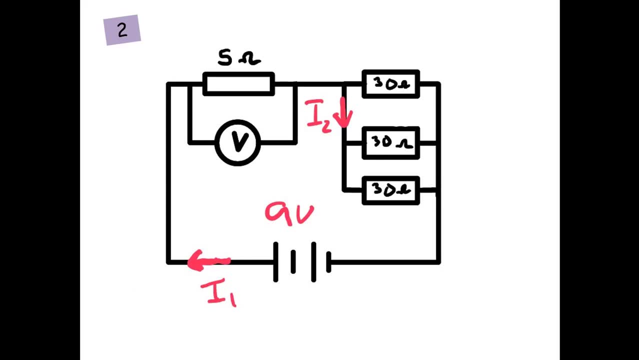 And we can find that I2 is 0.54 amps and I3 is 0.82 amps. Okay, Circuit number two. So I want you to try and find out what the total resistance of the 12 ohms is. 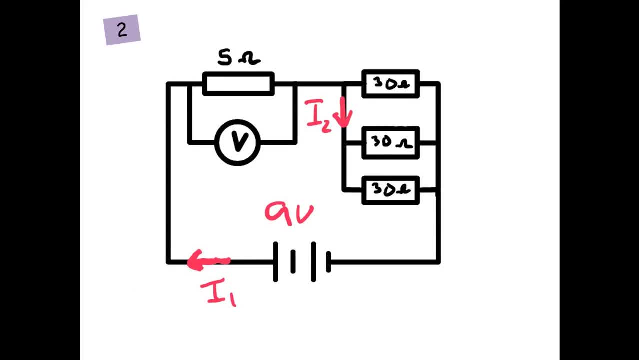 So we're going to try and find out what's the current I1,, what's the current I2, and then what's the voltmeter going to read as well. So pause the video now and try and have a go. 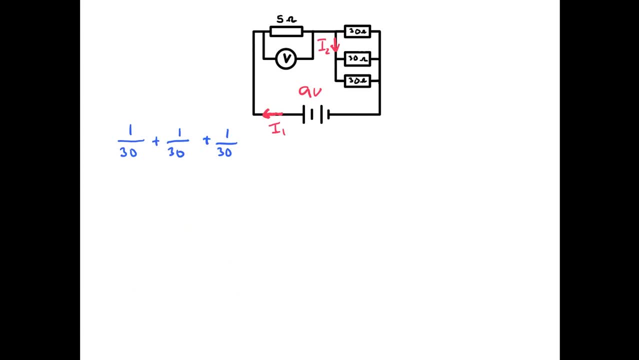 Okay, So here's my solution. Well, firstly, we've got those three 30-ohm resistors. They're all in parallel, So why don't we try and work out what their total resistance is? And we find that the total resistance is going to be 30 divided by 3, which is 10 ohms. 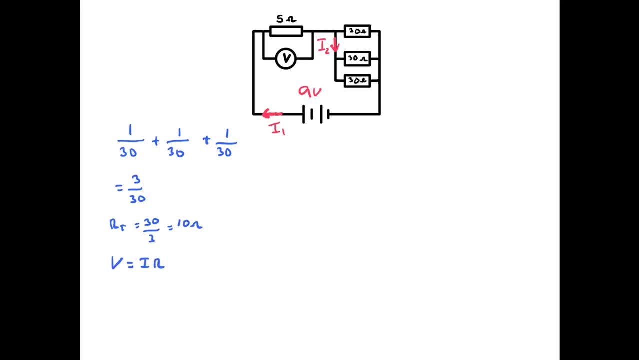 Then we're going to apply V equals IR. Now we know we've got 9 volts going into our circuit. We want to find that current I1. And then what's the total resistance? Well, we just worked out that those three 30-ohm resistors all in parallel is equal to 10 plus the 5 ohms. 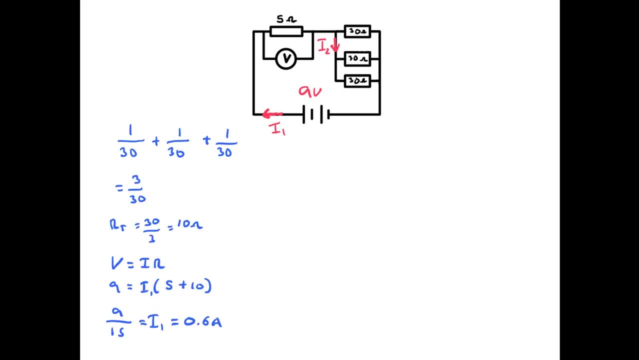 So I can add those all up together And I'm going to find the total resistance is 15 ohms. So 9 divided by 15.. 15 is going to give me my current I1, which is 0.6 amps. 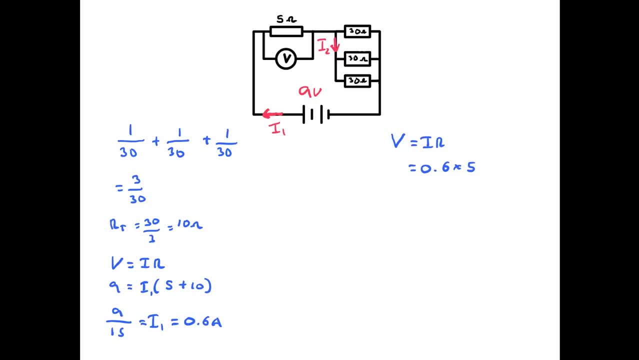 Okay, Now I can work out what V is going to be, Because if I've got 0.6 amps going through that 5-ohm resistor I can just apply V equals IR. So I know it's 3 volts across my 5-ohm resistor. 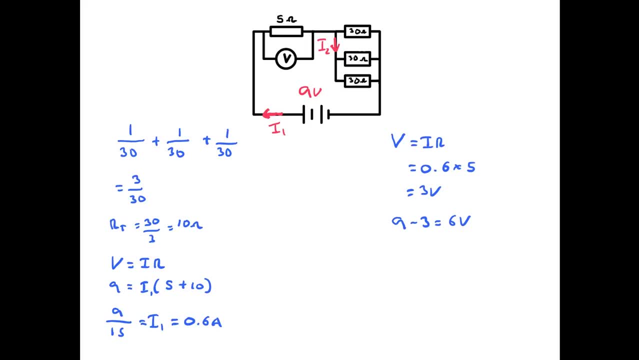 Therefore we must also have 6 volts across the 30-ohm resistors. Why? Because we've got 9 minus 3. It's going to equal to 6.. Now we know V over R equals I. So 6 divided by 30 is 0.2.. 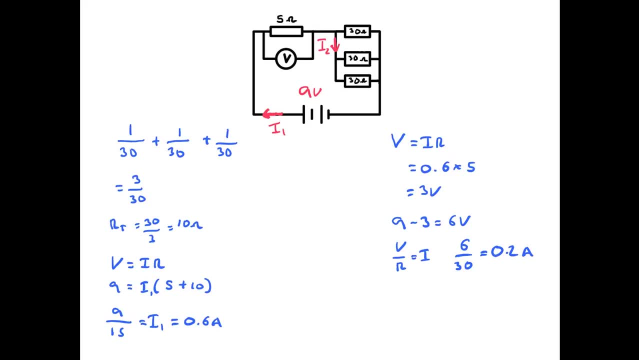 So in that very top resistor I know I've got 0.2 amps going through it. So if I know I've got 0.2 amps going through that top resistor and we know the total current going into the junction there is 0.6 amps. 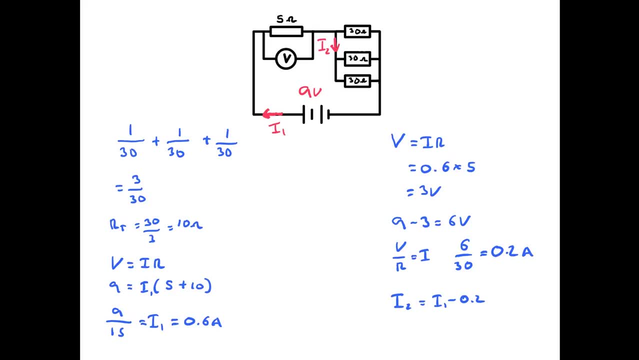 then the current going down is going to be 0.6 minus 0.2, which is going to be 0.4.. And that's going to be 0.2.. So that's going to be 0.2 amps. 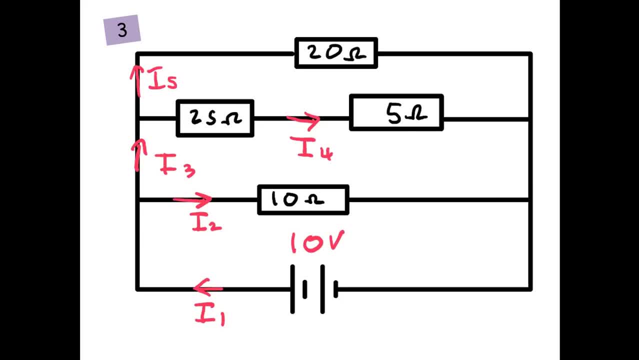 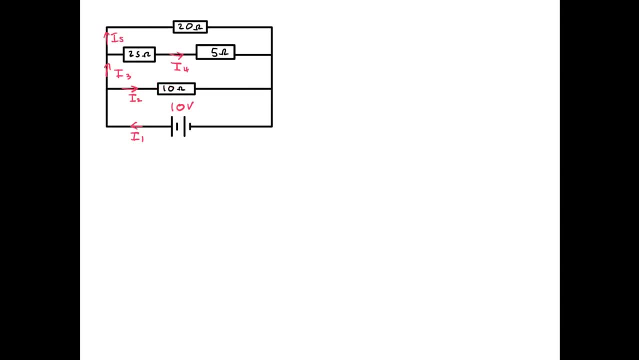 Okay, number 3.. I want you to try and find I1,, I2,, I3,, I4, and I5.. So try and draw the circuit and see if you can solve this problem. Okay, here's my solution. 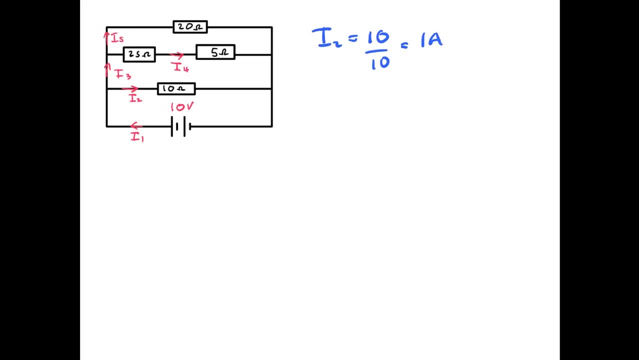 Well, firstly, we know that 10-ohm resistor that the current I2 is going through. well, that's going to have 10 volts across it because all our resistors, except for the 25 and the 5, are in parallel. 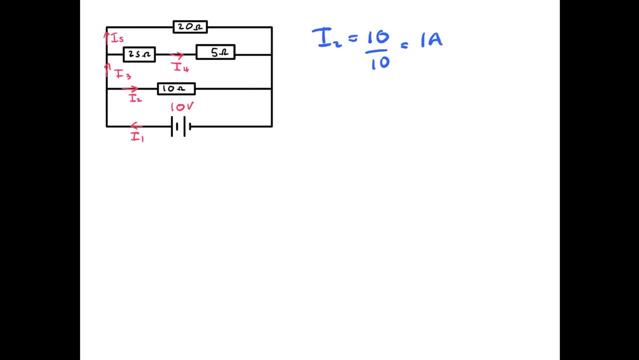 The 25 and the 5 are in series, but that whole section there is in parallel with the rest of the branches. Anyway, I2 is going to equal to 10 volts divided by 10 ohms, which is going to give you 1 amp. 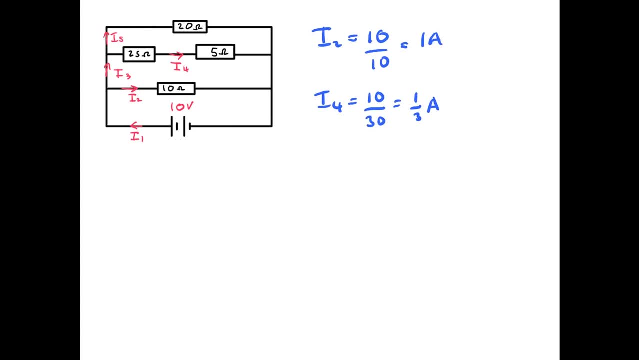 So now we've worked out I2.. Okay, well, what about I4?? Well, the total resistance in that branch is 25 plus 5, which is 30. So 10 volts divided by 30 ohms is a third of an amp. 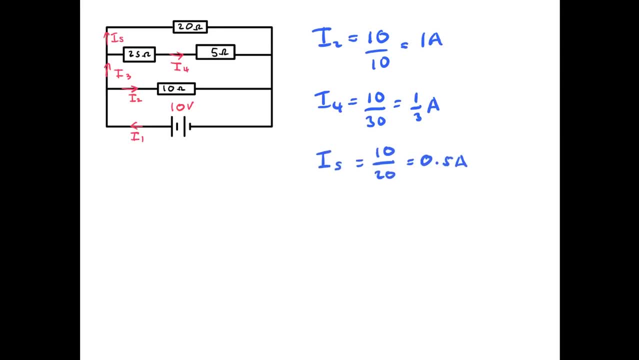 So that's I4.. I5, well, that's going to be 10 divided by 20, which is 0.5 amps. Okay, and now to work out I3.. Well, at that junction, I3 is going to equal I5 plus I4,. 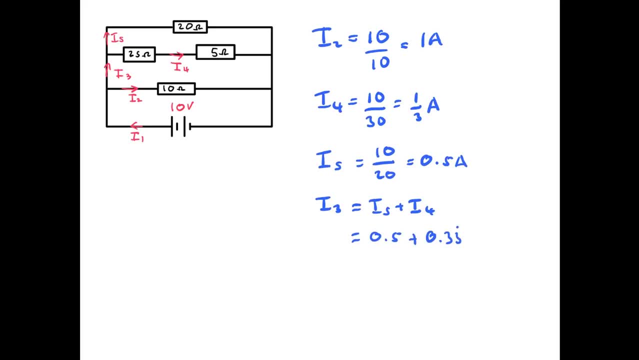 which we've both calculated them. So 0.5 plus 0.33 recurring, I get 0.83 recurring amps. Now I1 is going to equal I2 plus I3, and we both We know what those values are. 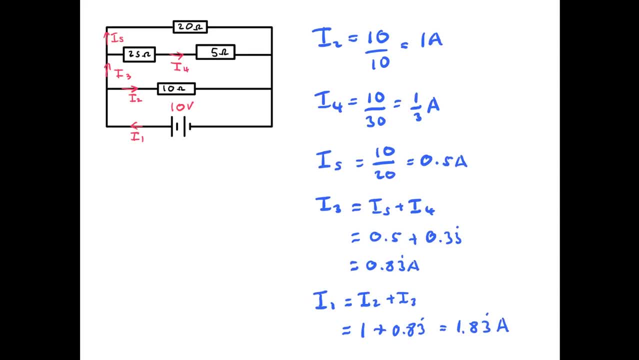 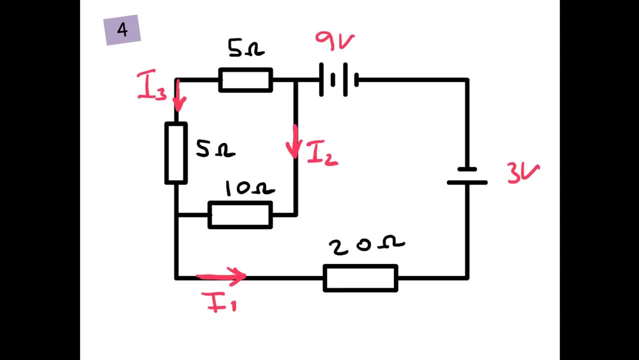 which is 1 plus 0.83 recurring, and we find that I1 is 1.83 amps. There we go. Okay, now, this time, be careful, because we've got two batteries, Well, a set of cells, which is 9 volts. 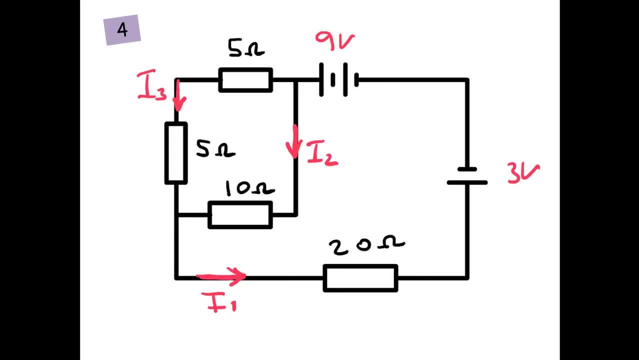 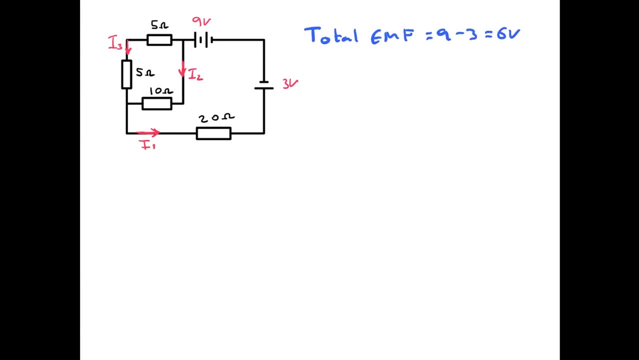 and then a cell that's giving out 3 volts. but be careful of the direction. I want you to Find I3 and I2, and then find me I1 as well. Okay, here comes the solution. Okay, so the total EMF is: 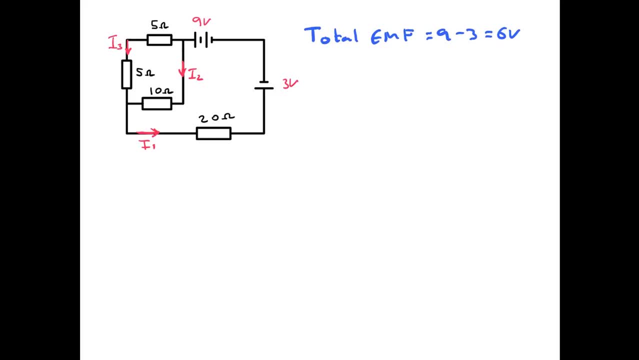 It's not 9 plus 3.. It's 9 minus 3, because the 3 volts is going in the opposite direction to the 9 volts. So the total EMF into our circuit is actually 6 volts. Now the branch with the two 5-ohm resistors. 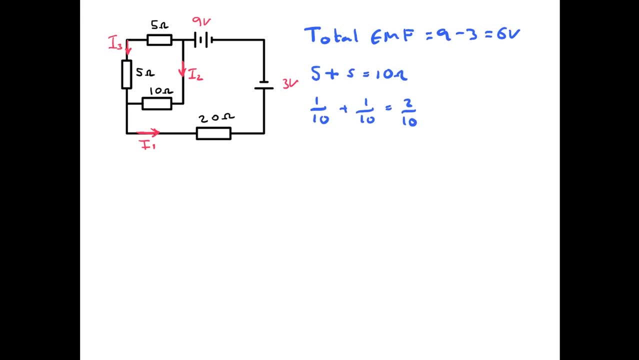 well, we can add those resistors up and we get 10.. And now we've got 10 ohms going one way, 10 ohms with the current going the other direction. So we can actually work out effectively. 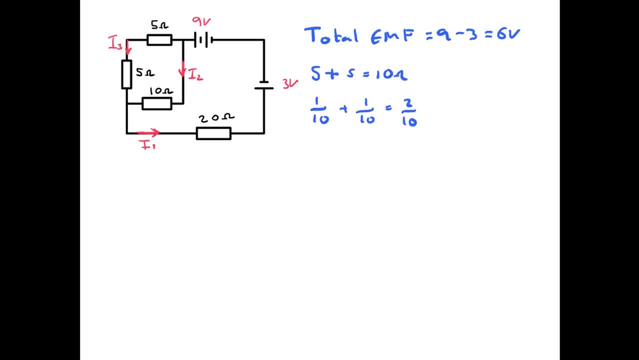 they're two sets of resistors in parallel. So what we can do is we can do 1 over 10, plus 1 over 10 is 2 over 10.. So that total branch in the left-hand side, or the 5 ohms and the 5 ohms and the 10 ohms. 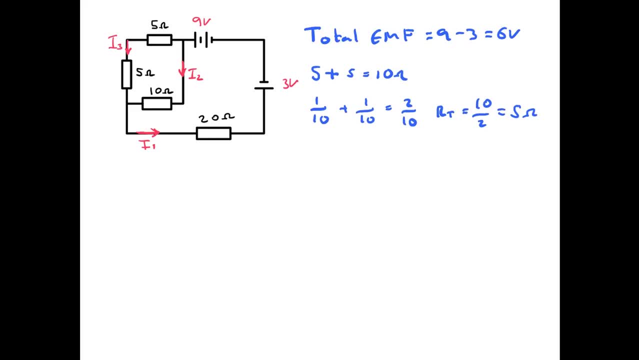 is actually all that resistor network there is actually equivalent to 5 ohms, And then we're going to apply V equals IR. Well, we know the total resistance now is 20 ohms plus the 5 ohms, So that's going to give us 25.. 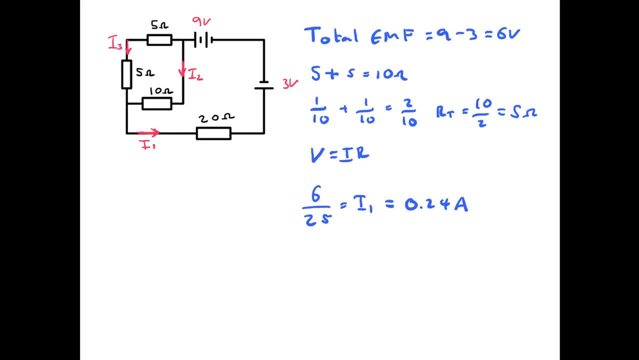 So 6 divided by 25 is I1, which is 0.24 amps. We know I1 equals I2 plus I3 at the junction. So we also know 10I2 is equal to 10I2.. 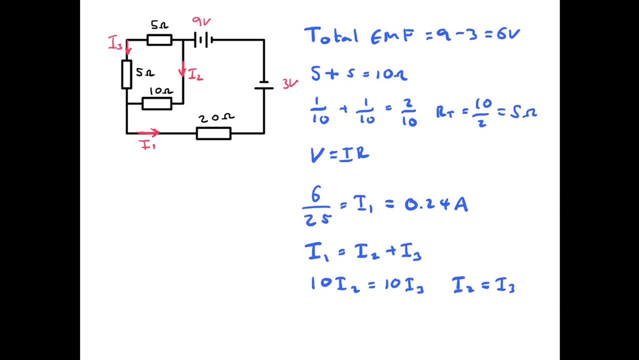 So we know 10I2 is equal to 10I3. Therefore, I2 must equal I3. So therefore, I2 and I3 must be half of I1. So half of I1 is 0.12 amps. 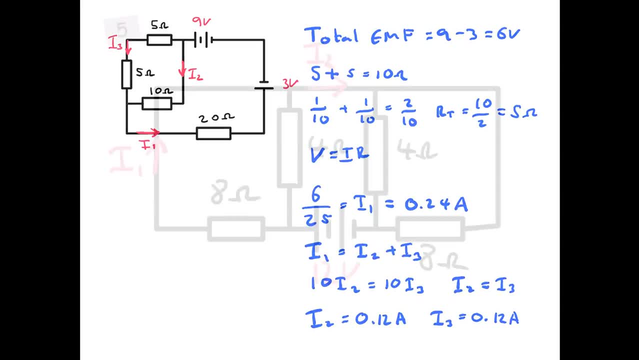 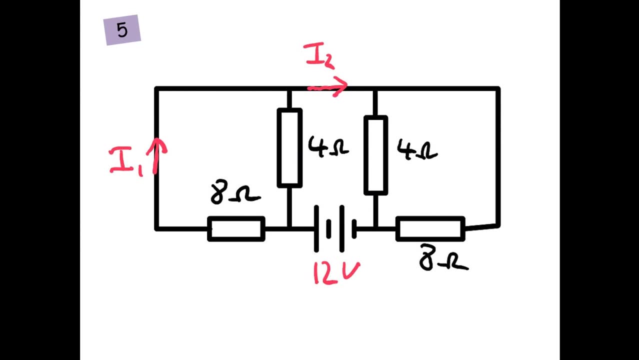 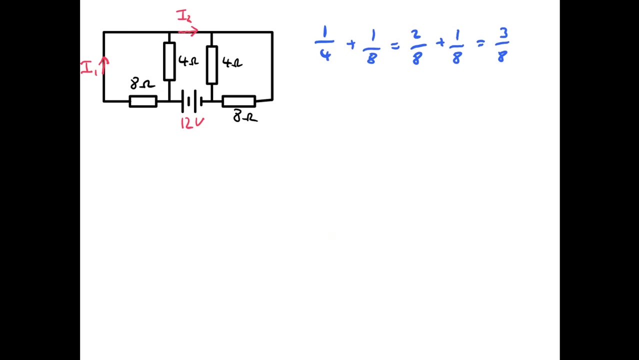 And exactly the same for I3.. Okay, number 5, our final little problem. So I want you to find I1 and I2.. Okay, here comes the solution. Okay, so firstly, we've got on the left-hand side. 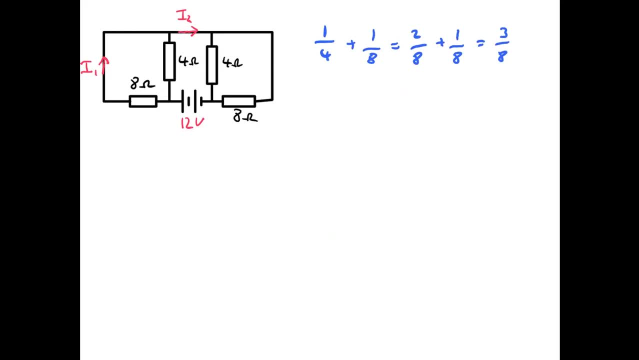 we've got an 8 ohm and a 4 ohm resistor in parallel So we can work out what the total resistance is there. So we can say: 1 over 4 plus 1 over 8 is equal to 2 over 8 plus 1 over 8,. 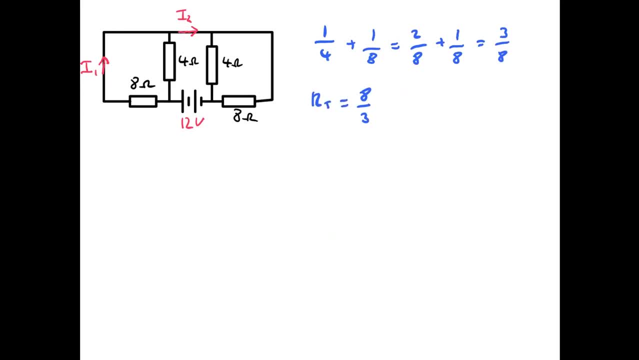 which is a total of 3 over 8.. We find the reciprocal of that, so that's 8 over 3.. And if you look, the resistor networks are actually kind of like a mirror image of each other, Because we've got an 8 and a 4 ohm on the left-hand side. 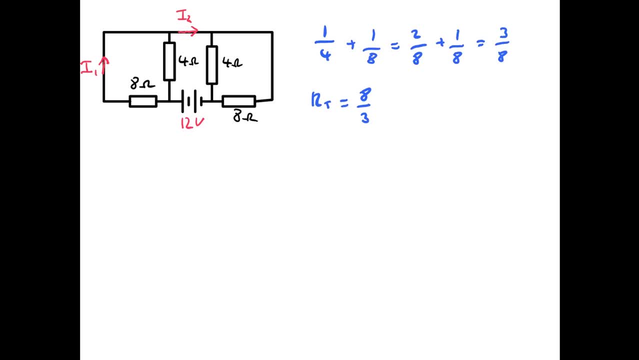 and a 4 and an 8 on the right-hand side, And the way they're connected is the same. So in fact, the total resistance is not going to be 0 over 3.. We can double it and that's 16 over 3,. 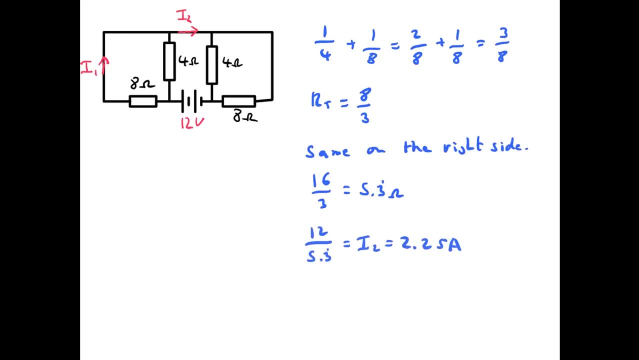 which is 5.3 recurring ohms. So now we can work out: well, what's the current going around our circuit? Well, that's going to be 12 divided by 5.3 ohms. That's going to give us I2, which is 2.2. 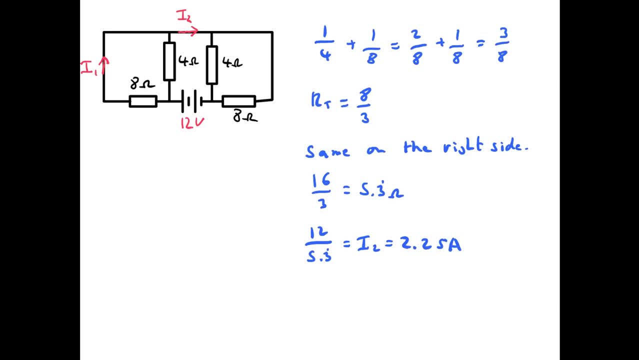 So that's going to be 0.25 ohms. Now what we need to work out is: well, what's the current for I1?? Now, this time, half the voltage is going to be going across the 8 ohm resistor.